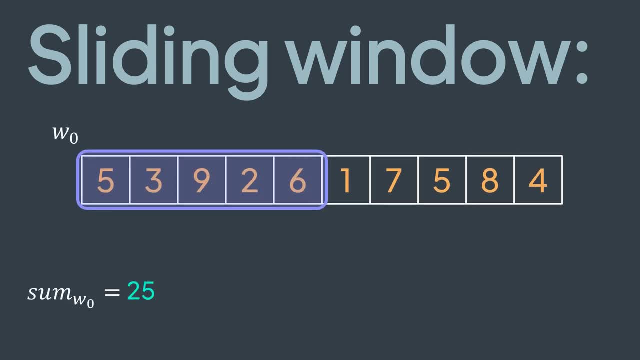 Quick example: we have this window and we know that the sum of its elements is 25.. If we want to get the sum of elements of the next window, we don't calculate the sum from scratch. we just take the sum of the actual window, add the new element, subtract. 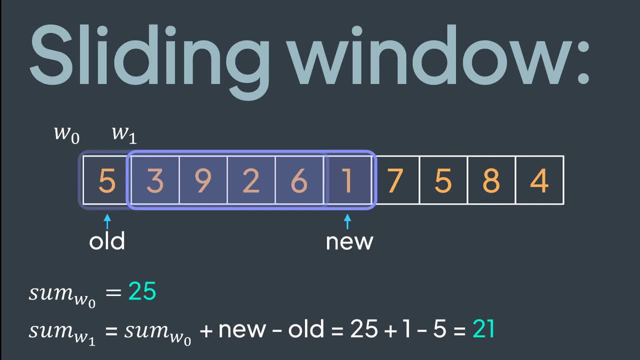 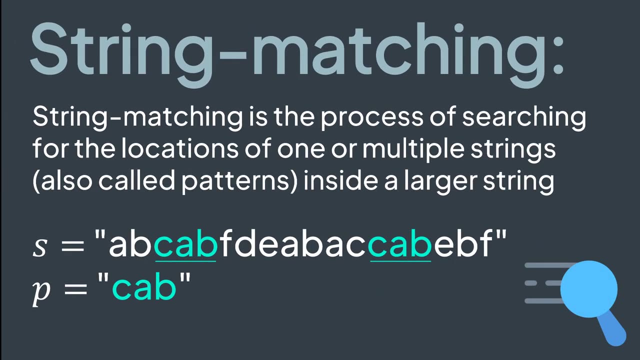 the old element and we got the new sum in all of one time. All of one, because the length of the window doesn't affect the number of operations. Last term, string matching. String matching is the process of searching for the locations of one or multiple strings, also called patterns, inside a larger string And there exists different. 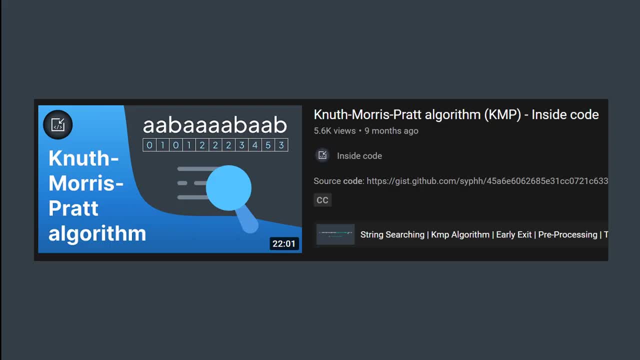 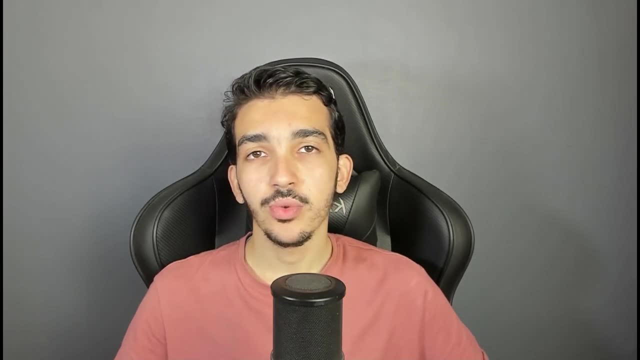 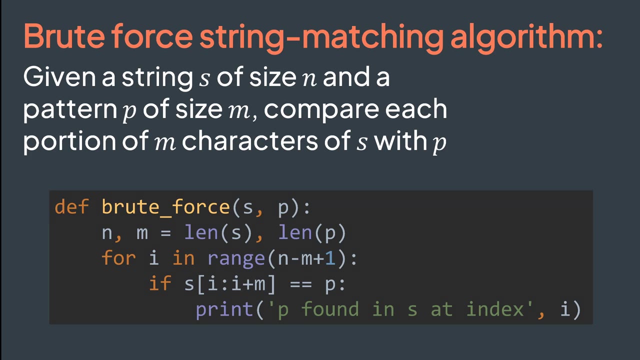 string matching algorithms. We've seen one in this channel, the KMP algorithm. We're now ready to start To search for a pattern in a string. there is a simple and straightforward way: the brute force algorithm. We have a string s of n characters and a string P of. 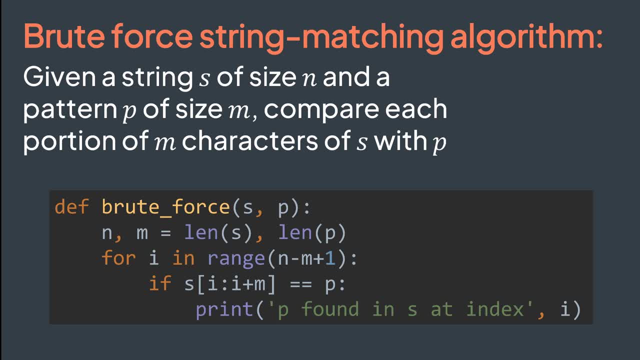 M characters. Two equal strings must have the same number of characters- M in this case, because we're searching for P. So the idea is to compare all substrings of s of M characters with P. We start from the beginning. we compare the. 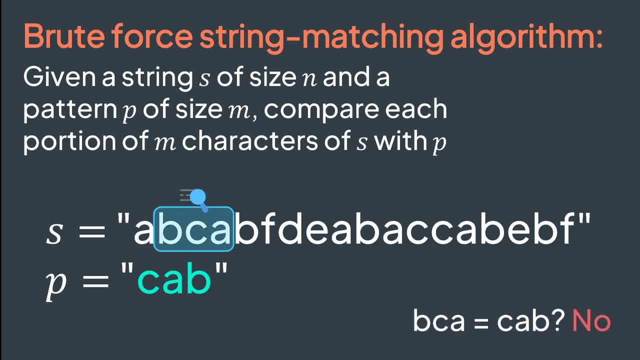 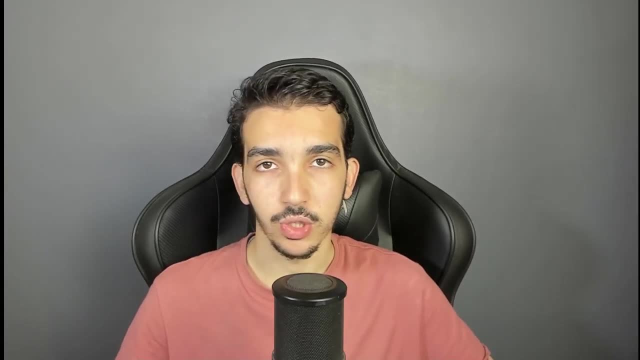 first M characters They don't match, Then the next M characters don't match, Then the next M characters they match. so we found P. We can continue like this to find all positions of P in s. You see very simple solution. Why don't we just use it then? Why would we use a more complex? 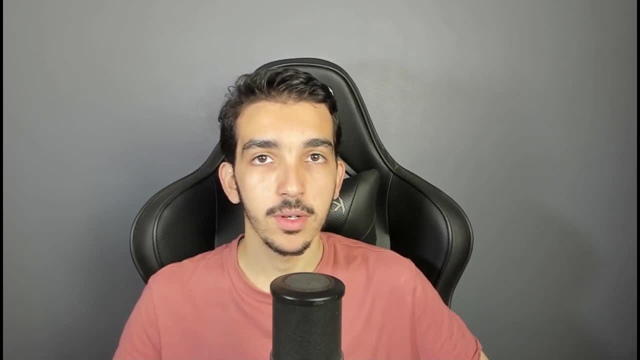 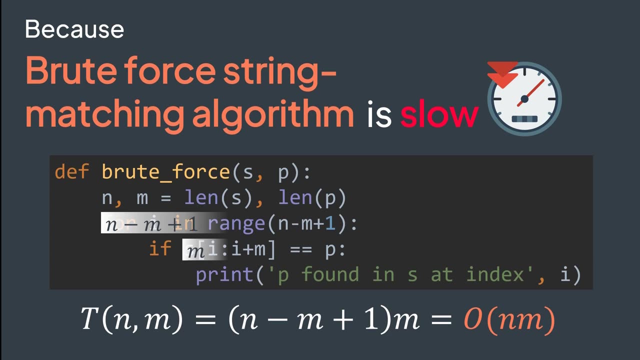 algorithm that uses hashing and sliding window. It's because the brute force solution is slow. Yes, what we're doing is that for each index in s, except the last ones, we're traversing the next M characters to compare them with P. 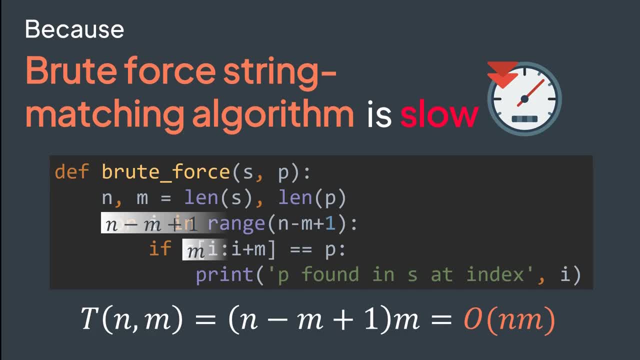 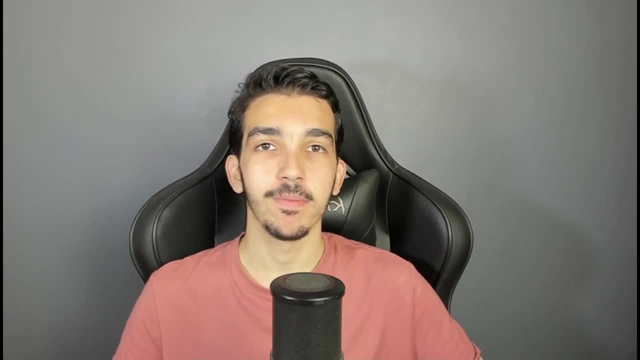 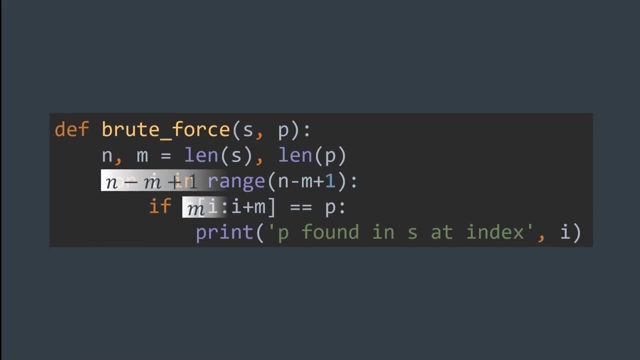 which gives a solution of O time complexity Quite slow, And this is why today we will learn about the Robin Karp algorithm. What's the idea of this algorithm? In the brute force solution, we have a loop that traverses indices of s and at each iteration we're comparing M characters, an operation. 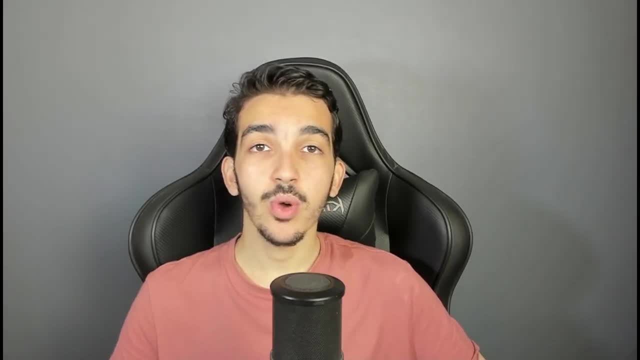 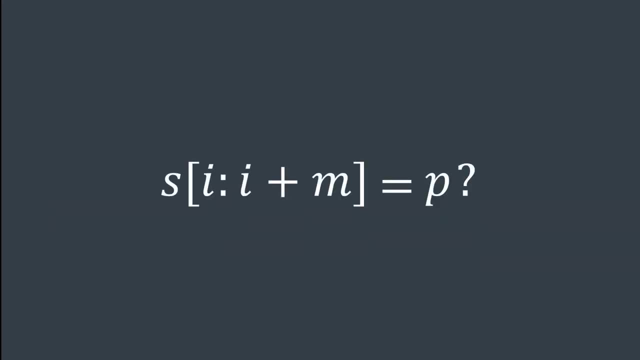 that costs O time, And this is what we want to eliminate. we want to get rid of this part. How to do so? The idea is that, instead of comparing strings themselves, we compare their hashes. In other words, by using hashing, we get the hash of each one of them, a fixed size, integer. 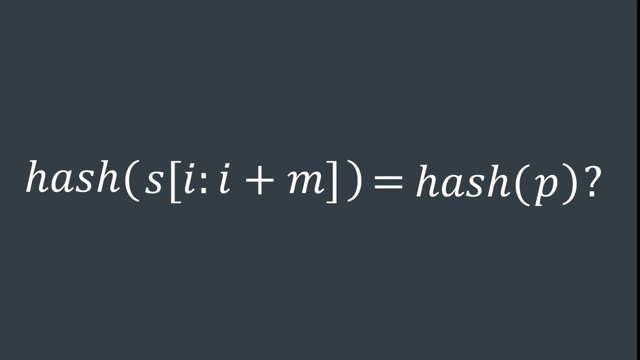 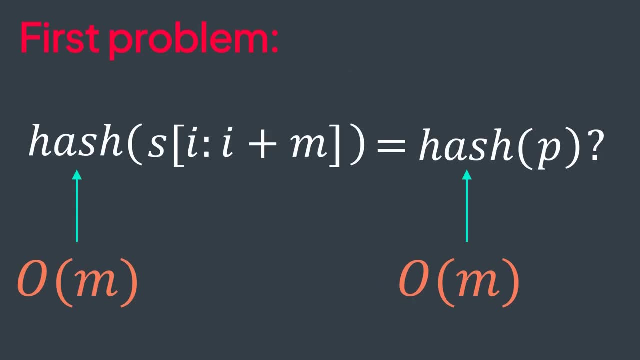 and we compare. The difference is that comparing integers is done in O time instead of O. But two problems arise from this reasoning. The first one is that calculating the hash of a string usually requires us to traverse the whole string, so it costs O in our case, which takes us back to our initial problem. 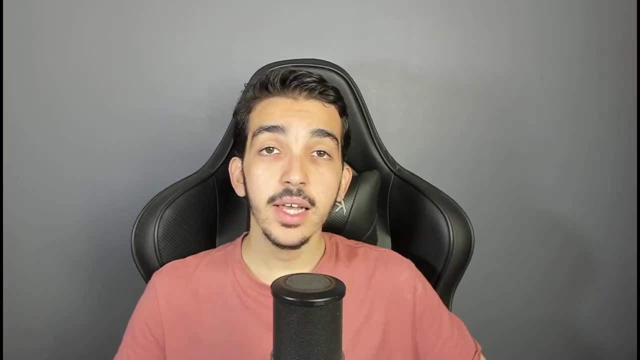 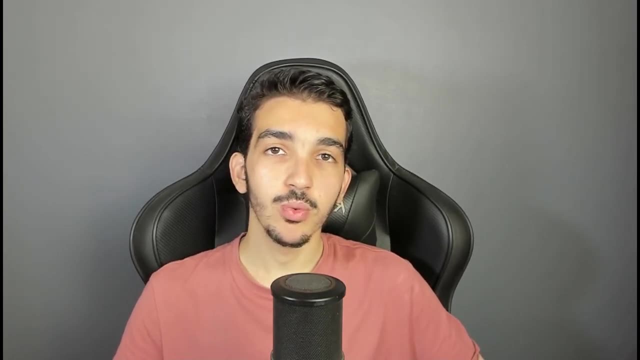 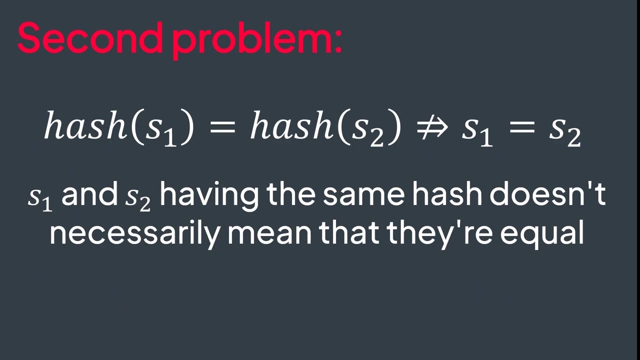 having our iterations running in O time. And second problem: having two strings with the same hash doesn't necessarily mean that they're equal. Remember the concept of collision we talked about in the hashing video? It means that saying that we found p as soon as hashes match can be wrong. this is why. 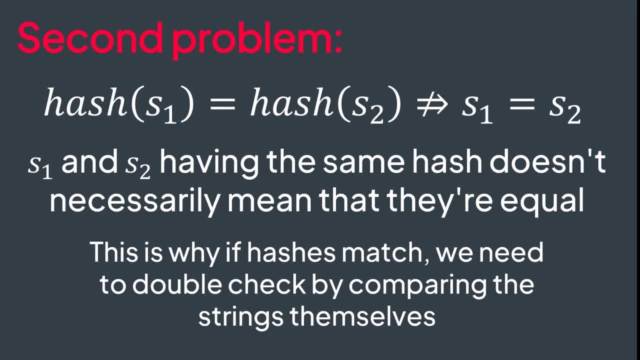 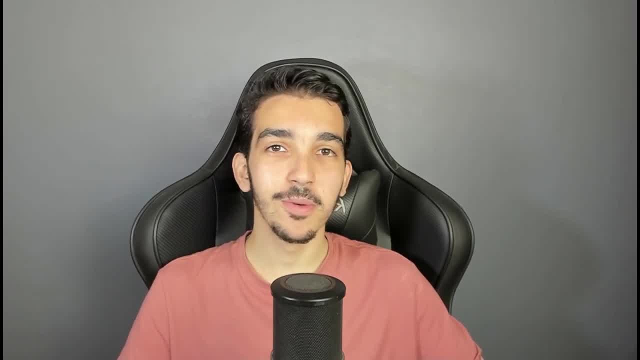 if hashes match, we get a hash of p. If hashes match, we double check by actually comparing the strings themselves before saying that we found p. I know this looks like we went back to the brute force algorithm, but with a more complicated. 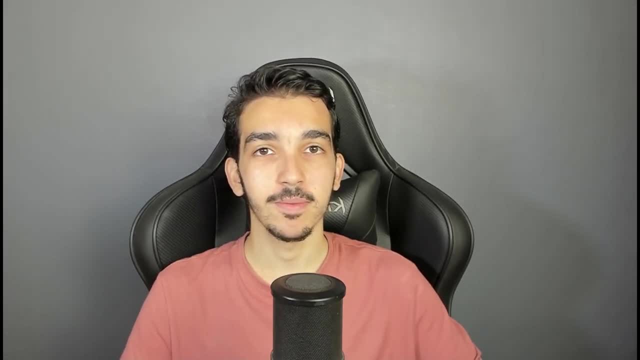 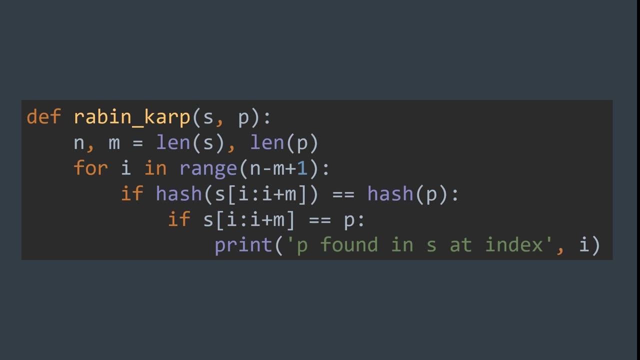 algorithm. But let's fix these problems. First, we said that calculating hashes takes O time because we need to traverse the whole string. Let's fix this. The pattern p doesn't change during the process, so we can calculate its hash once and store. 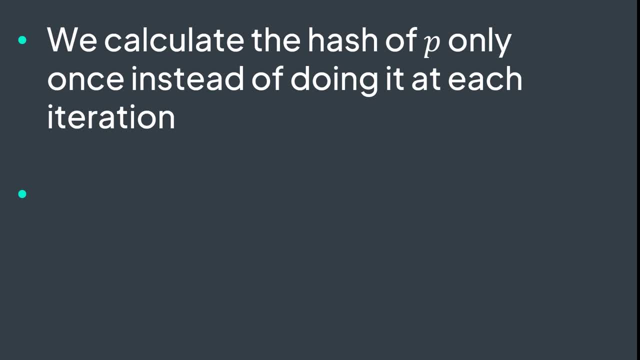 it in a variable. You don't need to do it at each iteration. And for substrings of s that we'll traverse windows, we will use the sliding window technique. We calculate the hash of the first m size window normally, then to get the hash of the 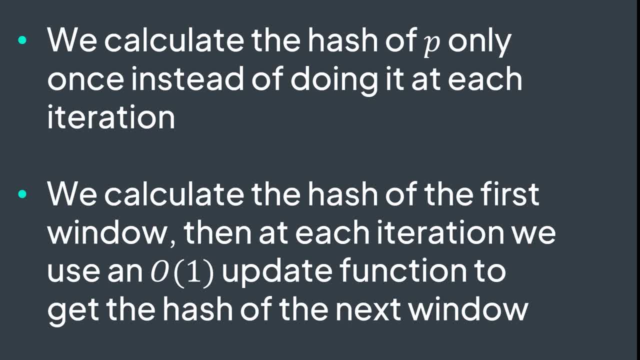 next window. we just update the actual hash by taking into consideration the character that entered and the character that went out. So getting the hash of the next window now costs O only instead of O. We don't need to traverse all the M characters again, we just work with the new one and the old one. 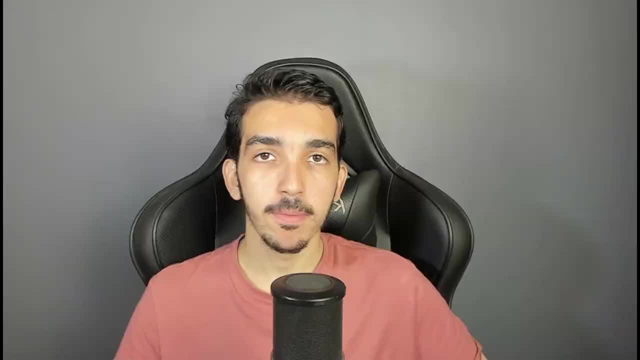 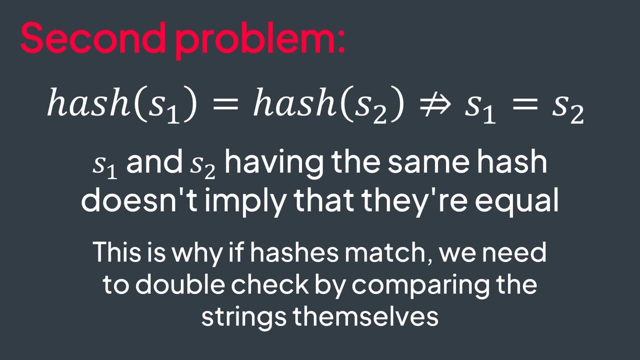 That was for the first problem we still have. the second problem is that two keys with the same hash doesn't mean that they're equal, which requires us to double check by comparing the strings, which is an O time. Can we have a hashing function that gives a unique hash to each key? 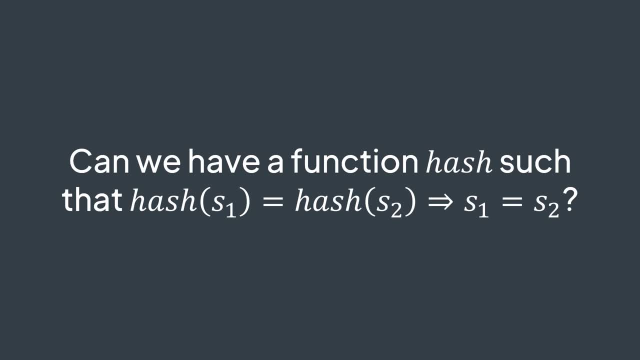 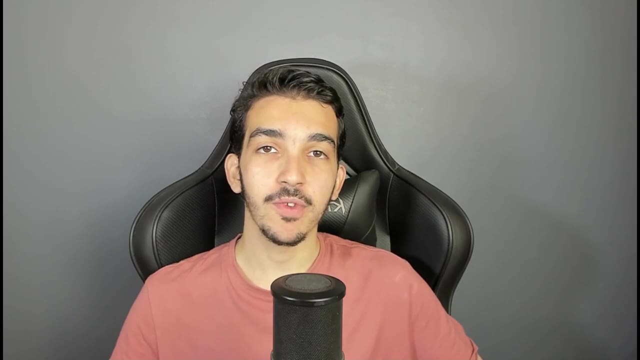 Because, if it's the case, we don't need to double check anymore. This is what we want. Well, this concept exists. It's called perfect hashing. We talked about it before, But because we have a huge number of possible keys, in our case it's impractical. However, we can still use a hashing. 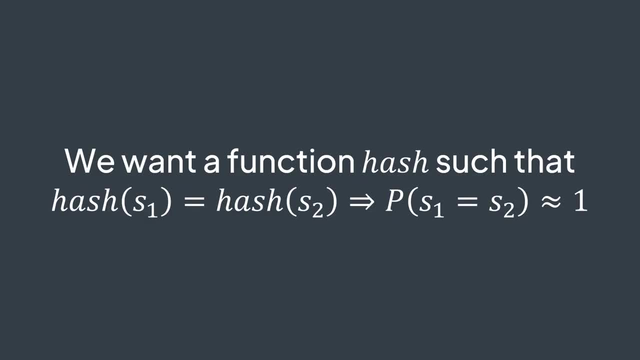 function that minimizes the number of collisions. we can use one that is good enough to say that if two strings have the same hash, we're almost sure that they're equal. the probability that they're equal is almost 100%. We still need to double check, but a good hash function will make us avoid. 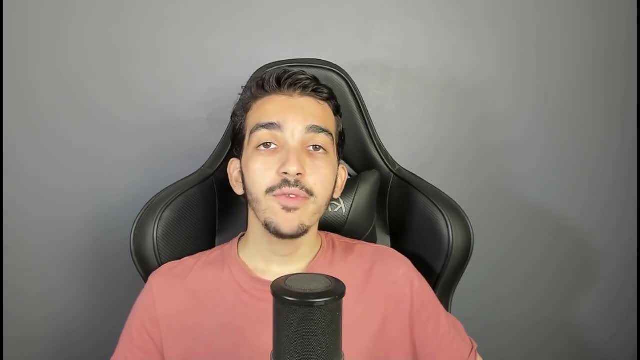 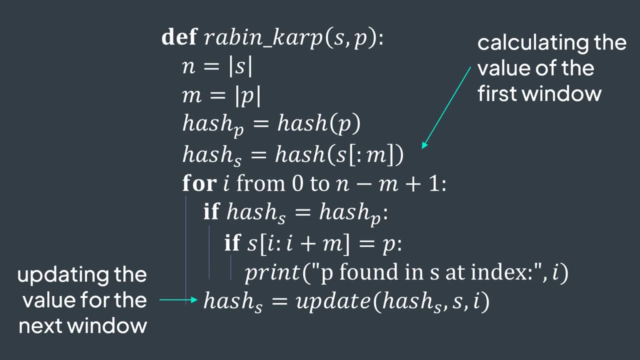 a lot of unnecessary problems. So let's go back to the first problem. Let's say that we have a hash of the first window that consists of the first key elements After introducing sliding window. here is our pseudocode In the maximum case. some example we've seen in the sliding 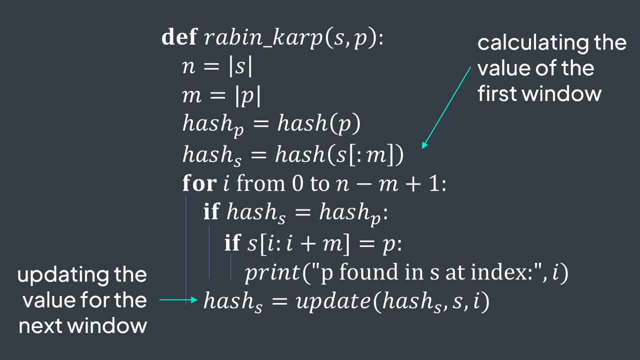 window video. we started by calculating the sum of the first window that consists of the first key elements. Then at each iteration we update the sum by using the new element and the old one to get the sum of the next window. We will apply the same logic here. we start by calculating the 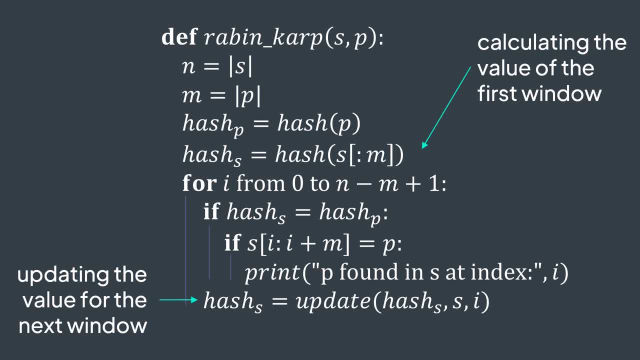 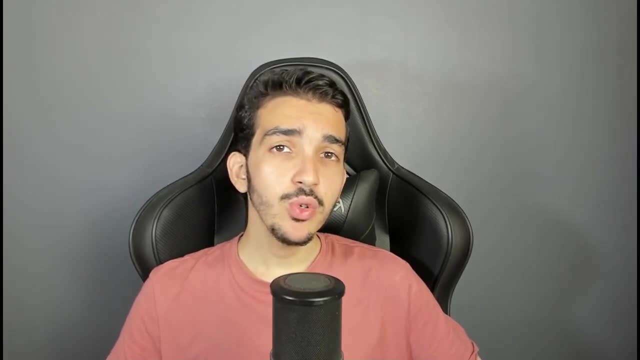 hash of the first window that consists of the first key elements. Then at each iteration, after comparing, we update the hash by using the new character that enters the window and the one that goes out to get the hash of the next window. But what do we use as a hashing function? As you may know, we have a lot of hashing functions. 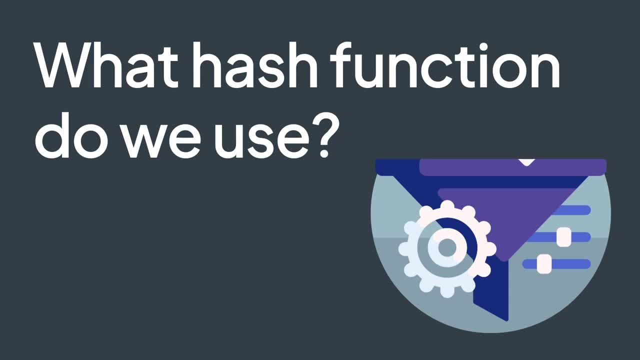 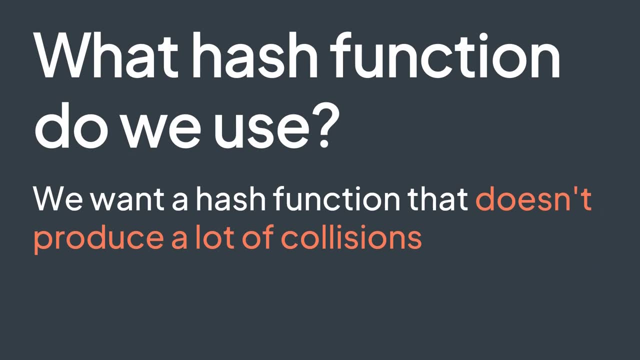 but we don't use any one of them. First of all, we want a hash function that doesn't produce a lot of collisions, to avoid unnecessary double checking. And second condition quite specific to our case, we want a rolling hash function, A hash. 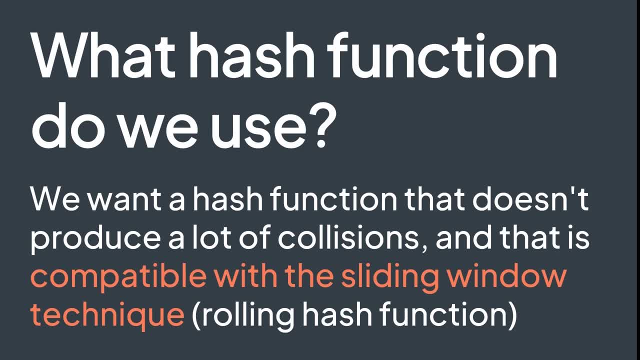 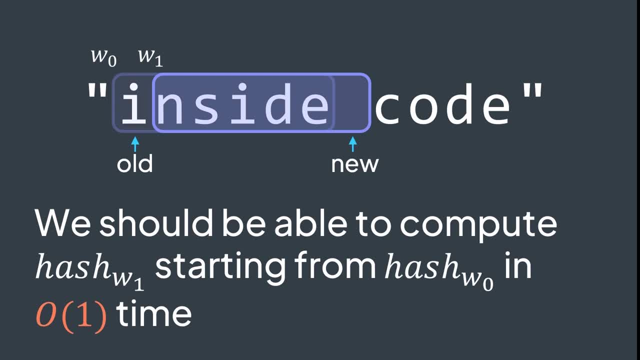 function that is compatible with the sliding window technique. It means that if we have two windows like this and we have the hash of the first window, we want to be able to get the hash of the second window without traversing old characters again. We want to get it just by. 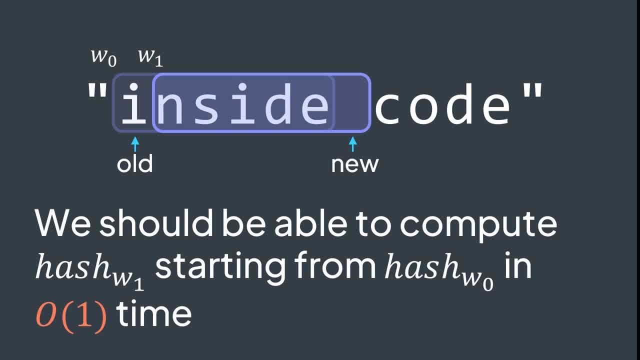 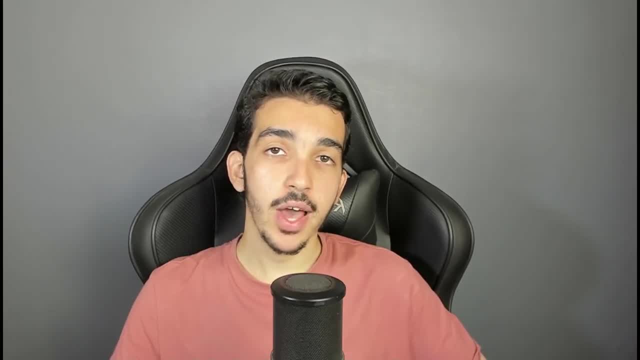 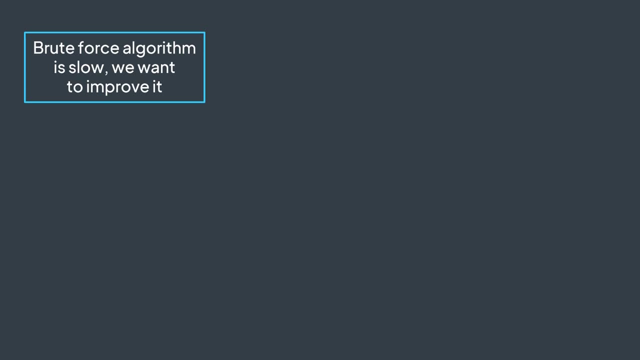 touching the new and the old characters To get hashes of next windows in over one time per iteration. A little recap before we dive into the hashing function we're gonna use. BruteForce solution has an O time complexity because it traverses M characters at each. 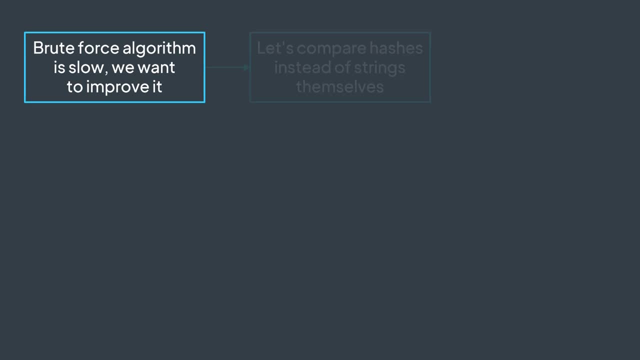 iteration to compare, To improve it. we want to compare hashes instead of strings themselves, because comparing integers is an O time But calculating the hash costs O, unless we use the sliding window technique with a rolling hash function to get the hash of the. 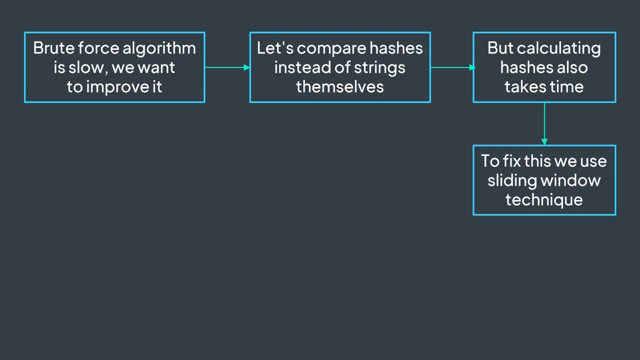 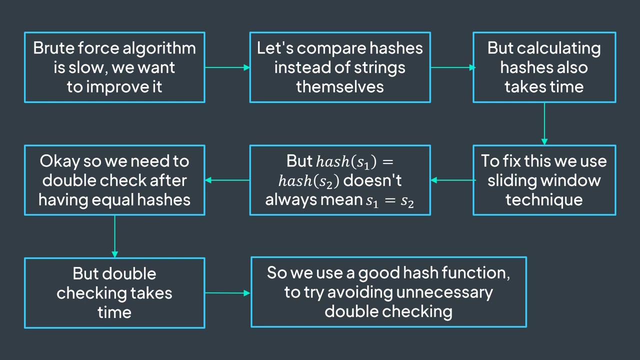 next window in O. Also, two strings with the same hash doesn't mean that they're equal. This is why we double check by comparing strings themselves to be sure, Which takes time. but by using a good hash function we reduce unnecessary double checking. 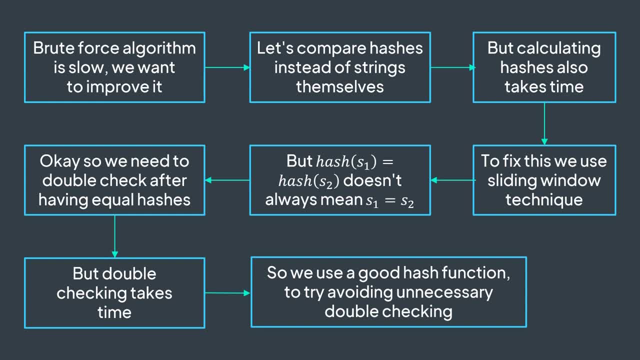 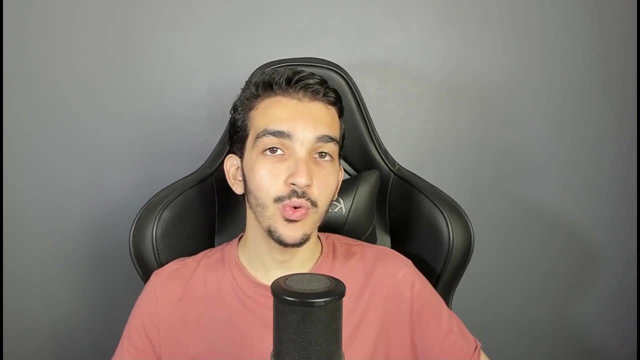 So, in brief, the robin carp algorithm optimizes the brute force algorithm by comparing hashes instead of strings and also uses sliding window to quickly compute hashes. If you understood this, you're quite good. Even so, we still need to understand two important things. 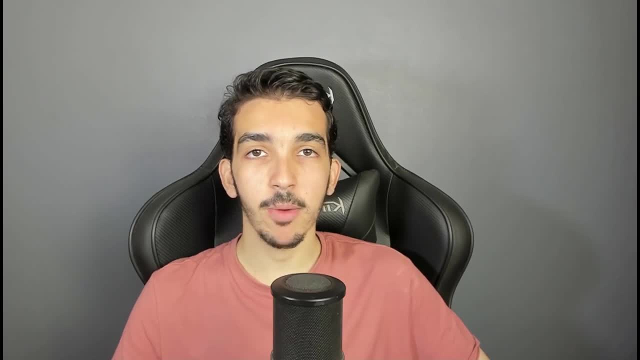 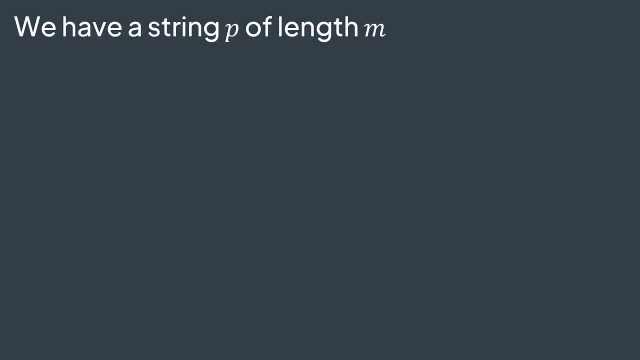 the hashing function we use and the time complexity of the robin carp algorithm. Let's start with the hashing function. Let's suppose that we want to hash a string p of M characters, like our pattern. For that we need two other variables, d, the alphabet size, and q, a prime number, to use modulo. 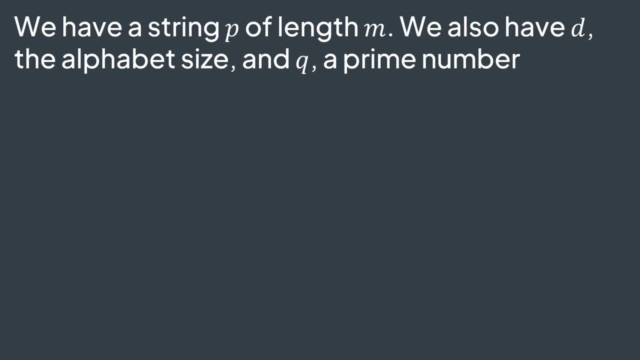 and avoid overflow. So we need two other variables, d- the alphabet size, and q- a prime number, to use modulo and avoid overflow. The alphabet size is the number of different characters our string can be made of. For example, if we're dealing with strings made of lowercase alphabetical letters only, 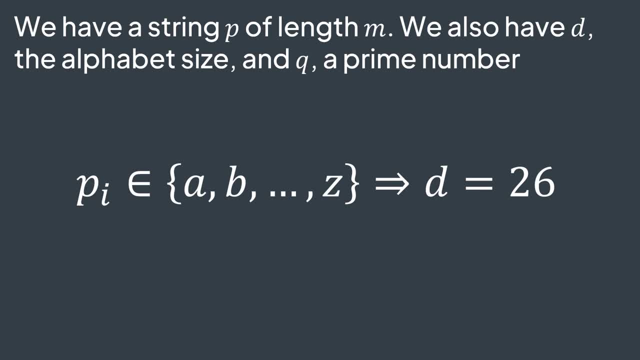 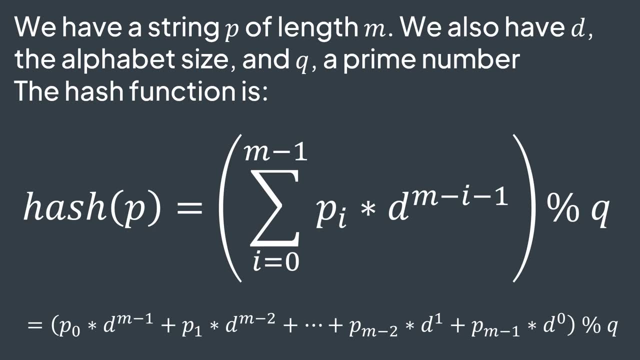 the alphabet size will be 26.. And the hashing function will be this one: the sum of the ASCII code of each character at index i multiplied by d, power, M minus i minus 1, all that modulo q. An example to understand. 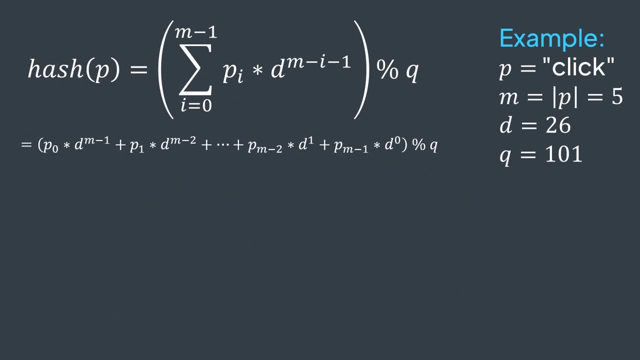 We have the string clique of 5 characters, so M is 5.. We also put d at 26, and q at, let's say, 101, it's a prime number. The hash of this string would be sk of c times d power 4, plus sk of l times d power 3,. 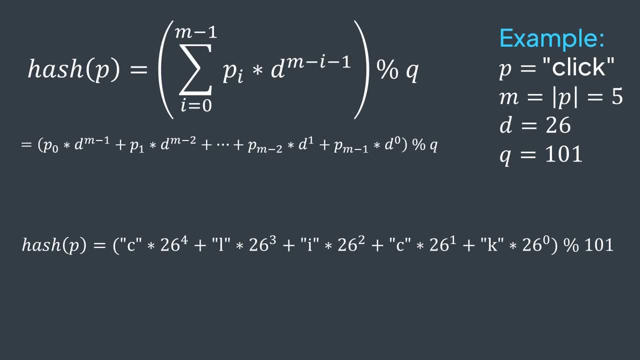 plus sk of i times d power 2, plus sk of c times d power 1, plus sk of k times d power 0, all that modulo 101, we get 43. So at the beginning we calculate the hash of p and the hash of the first window. 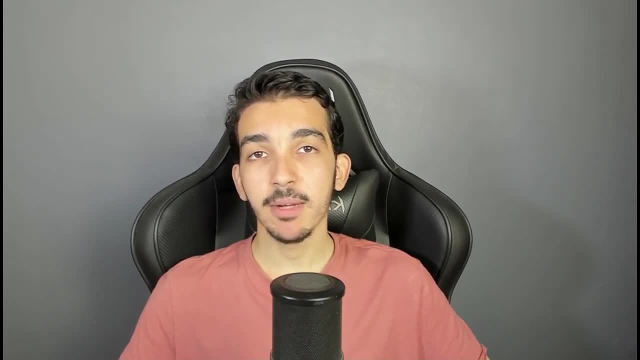 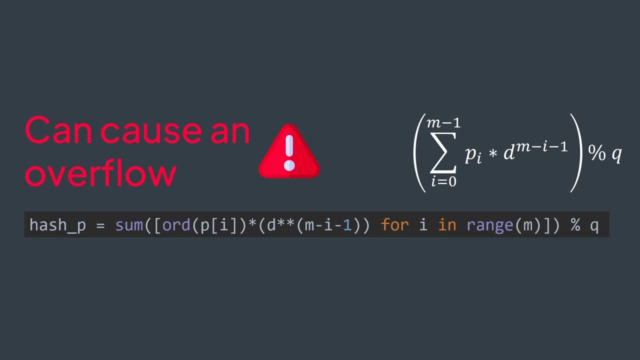 One small problem, however, is that because M and d can be quite big, calculating the sum can cause an overflow. To fix that and still get the same result, instead of calculating the hash of a key like this by directly calculating the sum. 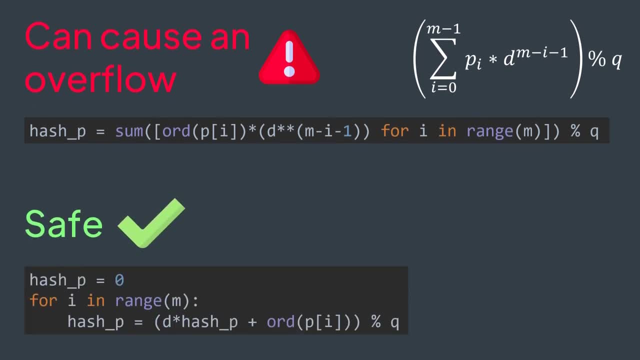 we write this: instead We start at 0, then for each character at index, i hash becomes d times hash plus i hash plus the sk code of the character. all that modulo q. You want the mathematical proof? Okay, fair enough. 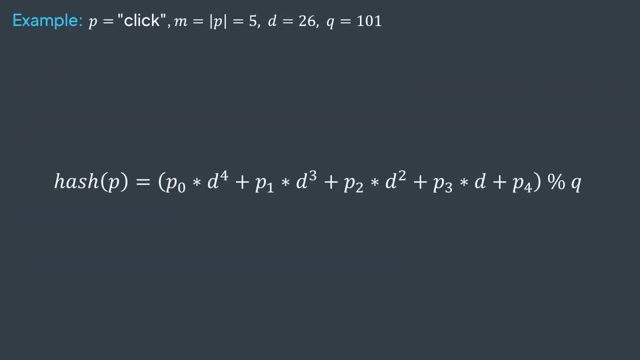 Let's stick to our 5 characters example. It's easier to understand than the general form. Actually, we're calculating the hash like this. right, Let's play around with this expression. You may know that d power k is equal to d times d power k minus 1, so we can factor by taking out d. 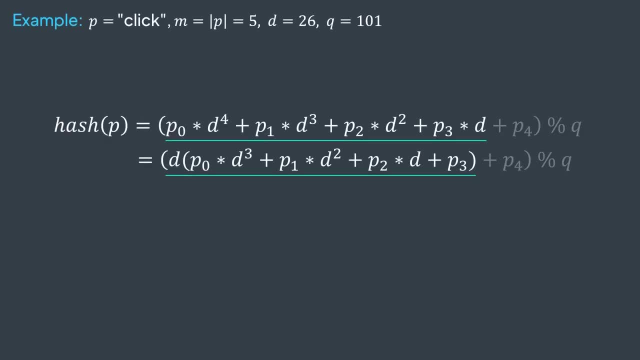 d. Here we do it for the first 4 terms. We have d times p0 times d power, 3 plus p1 times d power 2 plus p2 times d power, 1 plus p1 times d power 0. By the way, d power 1 is. 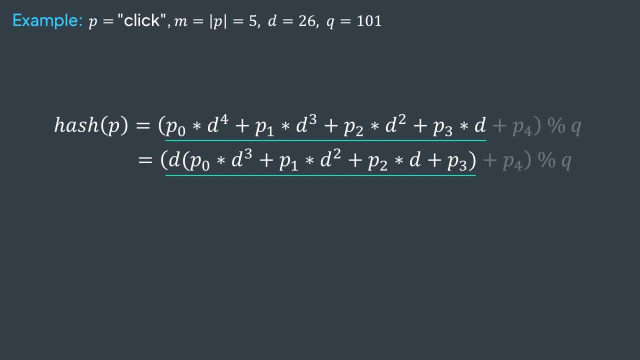 d and d power 0 is 1.. Now we factor the first 3 terms, We get d times p0. times d power 2 plus p1. times d power 1 plus p2. times d power 0.. Now we factor the first 2 terms, We get d times d times power 0 plus p1.. And we just 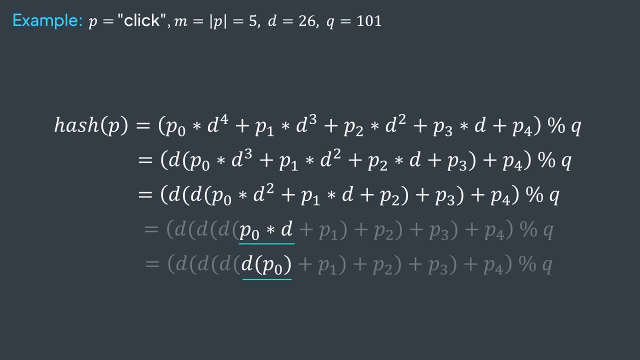 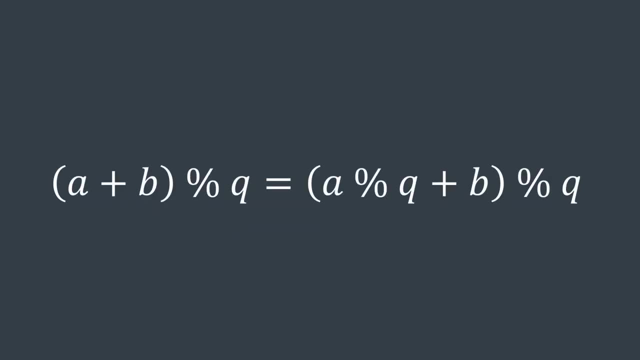 put parenthesis like this: Okay, now we got this expression. You need to know that a plus b modulo q is equal to a modulo q plus b modulo q. Also, d times a modulo q is equal to d times a modulo q By combining these 2 laws. 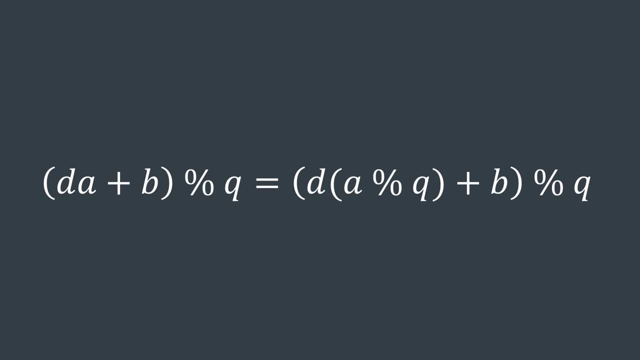 we get that d times a plus b modulo q is equal to d times a modulo q plus b modulo q. And we use this law to introduce modulo q like this: by considering d, a and b, like this. Same thing here, by considering d, a and b, like this, we can introduce modulo q. We do. 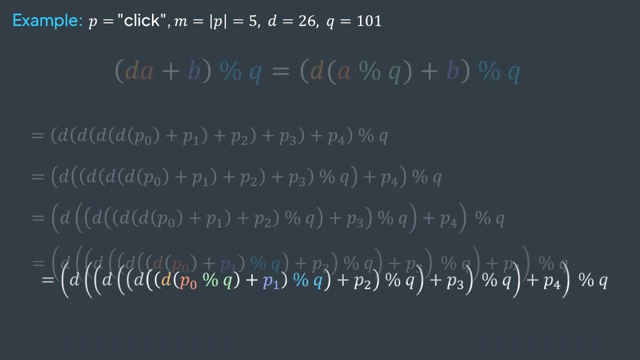 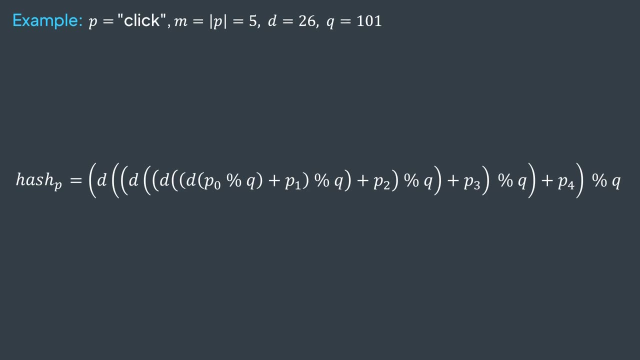 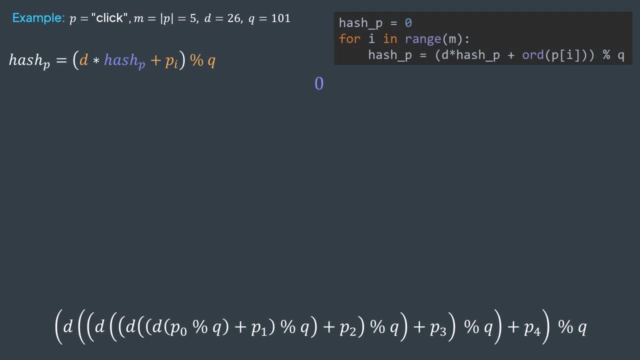 it again here and we do it again here, We get this expression: Well done Bye. Last thing: how to compute this expression. Remember that this expression represents the hash of p. we can do it like this: hash p starts at zero, then we multiply it by d, add p zero. 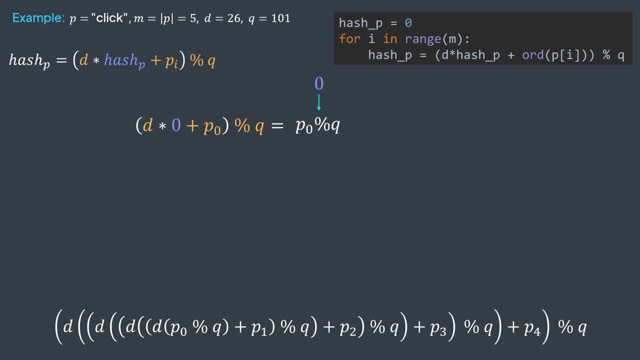 all that module q, we get a new value. Then again we multiply it by d add p. one, all that module q. Again we multiply by d add p. two, all that module q, And again, multiplied by d, add p. three, all that module q. Again, multiply by d add p for all that module q and we get the hash. 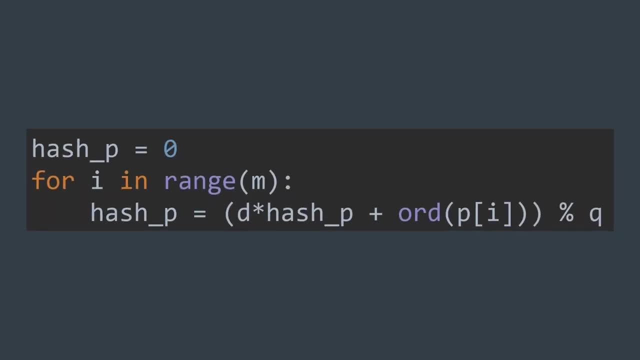 And if you noticed, what we did here is that hash p started at zero. then for each character hash p became D times hash p plus pi, all that module q, And this is why we could avoid overflow by turning our sum into a sequence of safer. 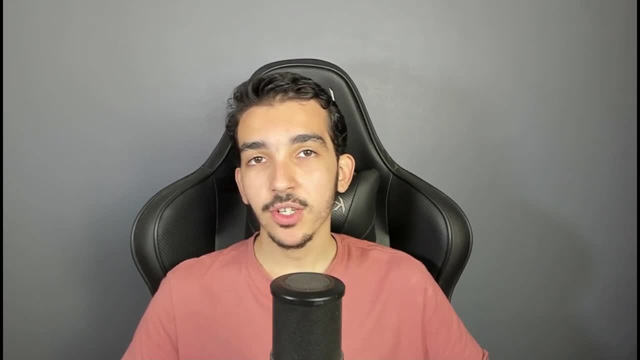 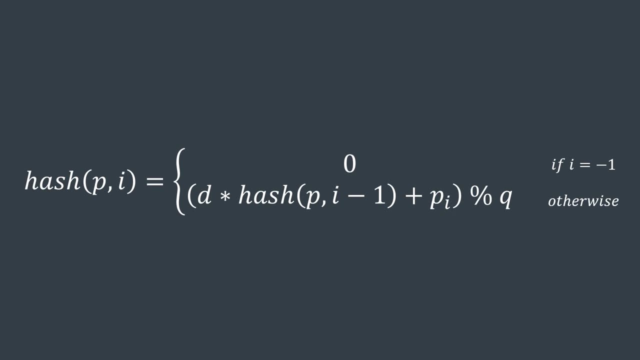 operations. We can even define our hash function as a recursive function, hashing characters of p until index i is equal to zero. if i is minus one, it means we finished hashing. and D times hash of i minus one plus pi, all that module q else. Okay, now we know how. 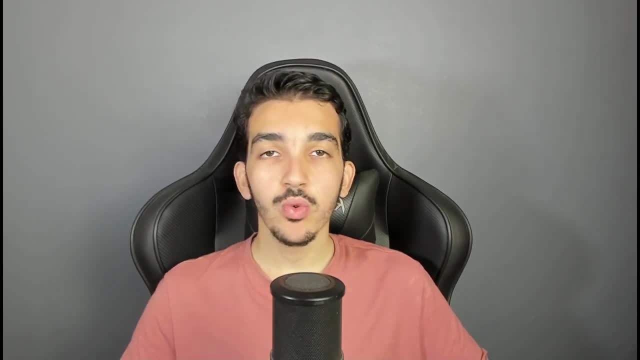 to compute this expression. Let's see how we can compute this expression. Let's see how we can compute this expression. Let's see how we can compute this expression. Let's see how to hash while avoiding overflow. We use what we made now to hash p and the first M characters of s. 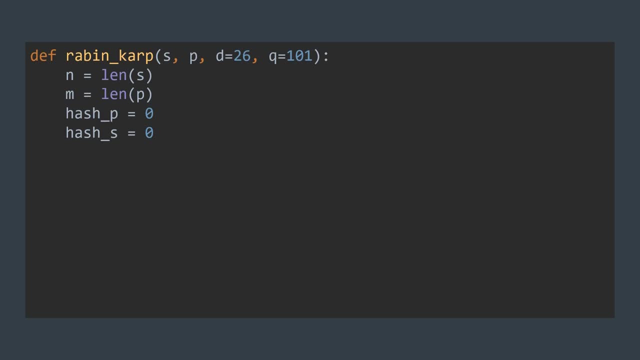 In code we will have two variables: hash p and hash s. Then we traverse the M first characters of s and p while performing the operation we've seen now Hash p becomes D times hash p plus sk of pi. module q. Same logic for hash s. Next step we can start traversing in this: 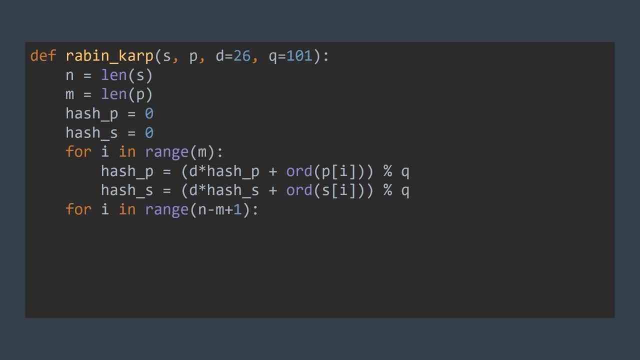 way We can compare the M characters of s to compare and update. First we compare. We compare the hash of our window hash s with the hash of our pattern hash p. If they're equal. we double-check by comparing strings themselves. We compare the. 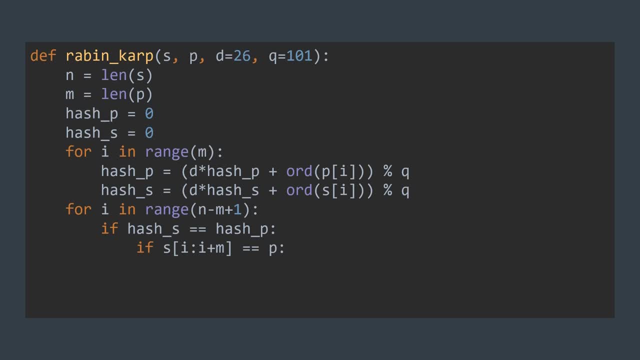 next M characters of s starting from i with p, If they're equal. then we found p in s at the index i. That was for comparison. But what about a new hash? We need to update hash s for the next window by removing the old character s of i. 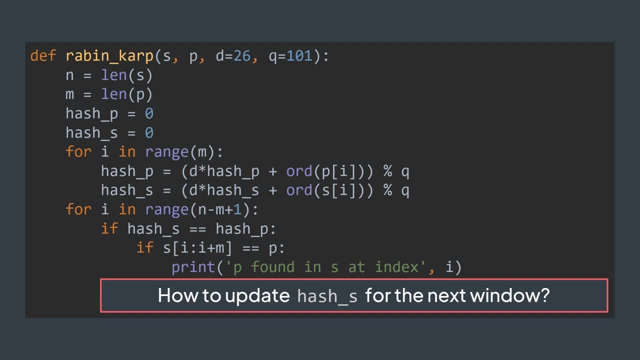 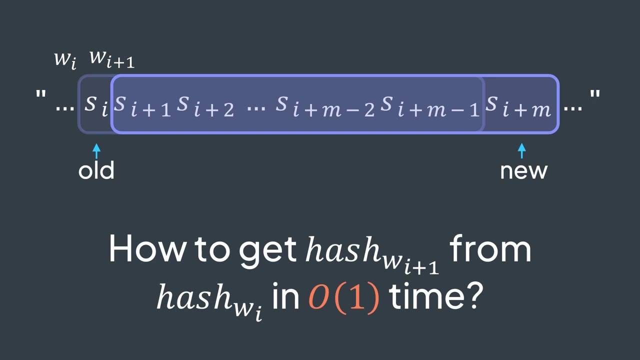 and adding the new character s of i plus m. Yes, we can just calculate the hash again from scratch, but we don't want that. We want to go from the hash of the window i to the hash of the window i plus 1 in O time. Let's take this example and get ready for another mathematical demonstration. 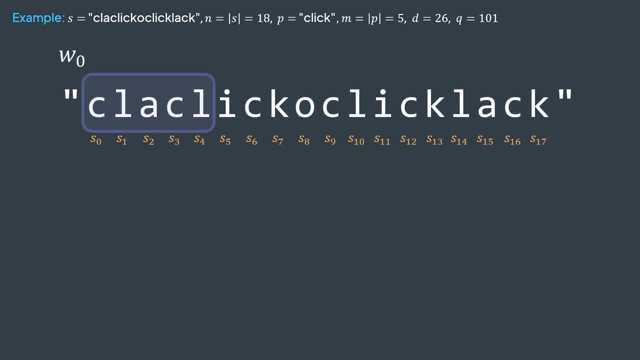 Here M is 5, so our first window consists of the first 5 characters of s. Let's calculate its hash: It's s0 times d power 4 plus s1 times d power 3 plus s2 times d power 2. 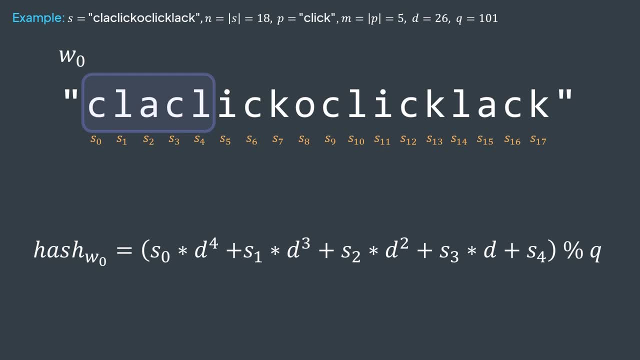 plus s3 times d power, 1 plus s4 times d power, 0. All that modulo q. What about the hash of the next window, the one that starts at index 1? It's s1 times d power, 4, s two times d power, three plus s three times d power, two plus s four times d power, one. 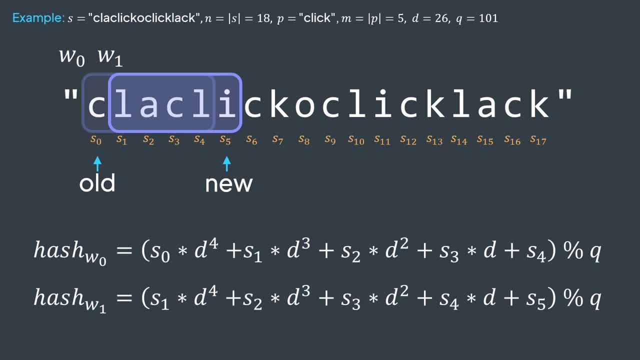 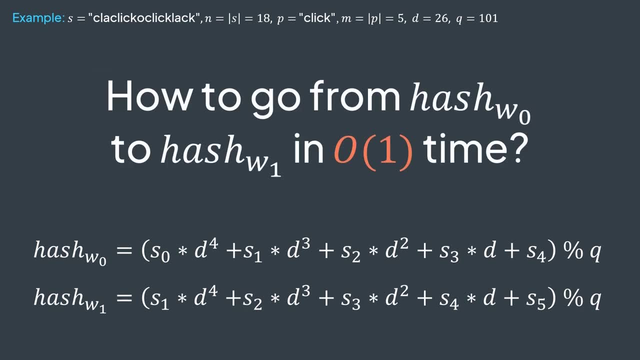 plus s, five times d power, zero. all that modulo q. We want to go from this one to this one in all one time. how to do so? First of all, we can notice that, as zero times d power four is not present at all. below is the character that went out. we want to remove it from the. 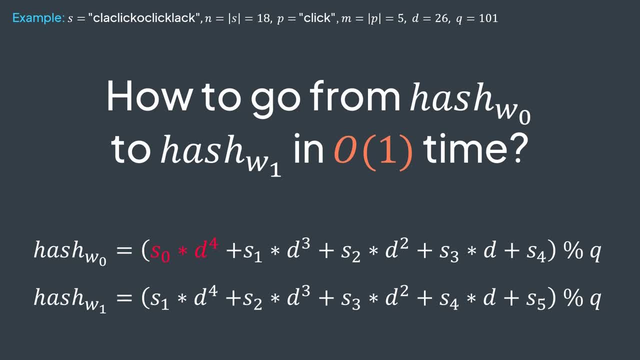 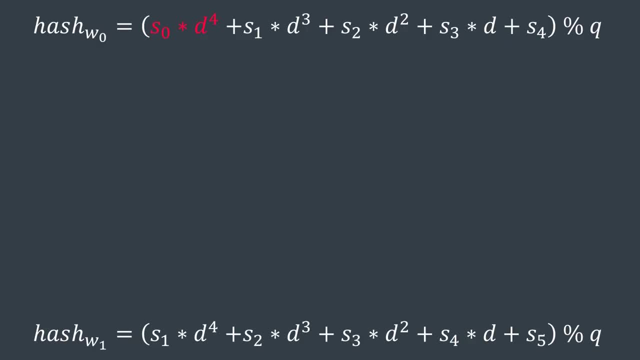 sum. But we don't remove it just like this. Notice that all this expression is modulo q. we have to respect modulo arithmetic laws. We have that a plus b, modulo q minus a, all that modulo q is equal to b modulo q. By putting a and b like this, a gets removed, a is s. 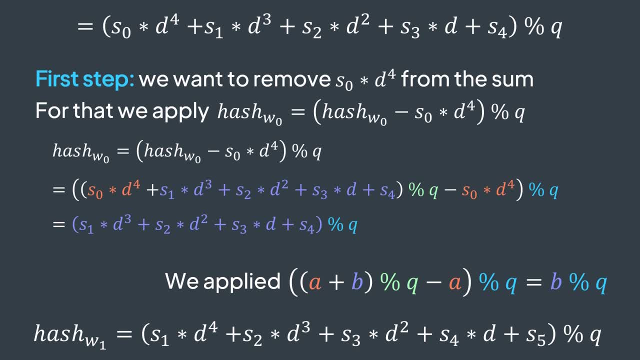 zero times d power four. So by subtracting it and putting the result modulo q and using the law, we'll get b modulo q. So by subtracting it and putting the result modulo q and using the law, we'll get b modulo q. 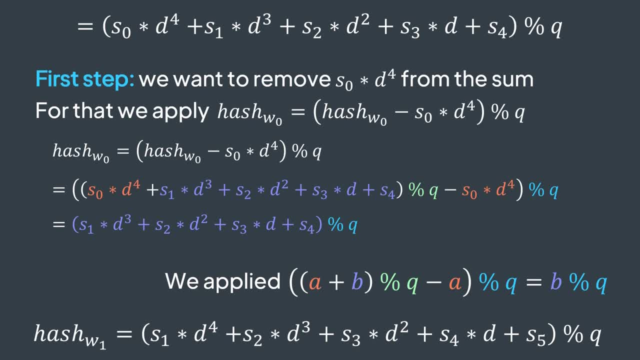 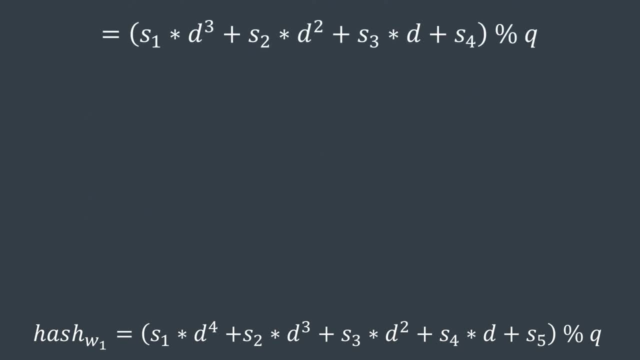 Where b is the sum, but without the first term. Next step: we notice that powers have to be incremented to reach those in the expression below. For example, now we have s one times d power three, but in the final expression we have s one times d, power four. To increment all powers, we multiply everything by d and 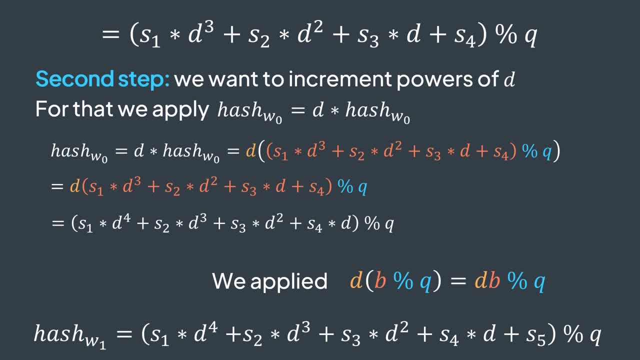 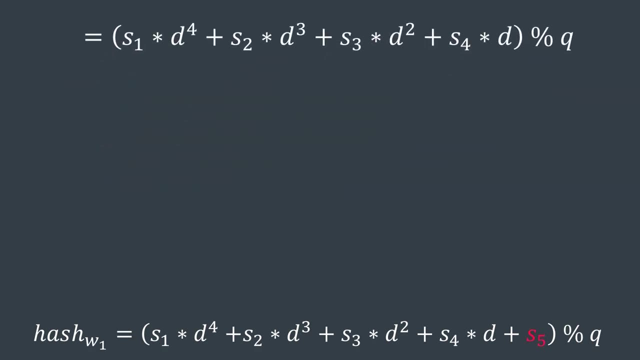 apply this law: d times b modulo q is equal to d times b modulo q, where b is our actual expression. You can see that now powers match. Last difference: we don't have s five, we have to add it. it's the new character. 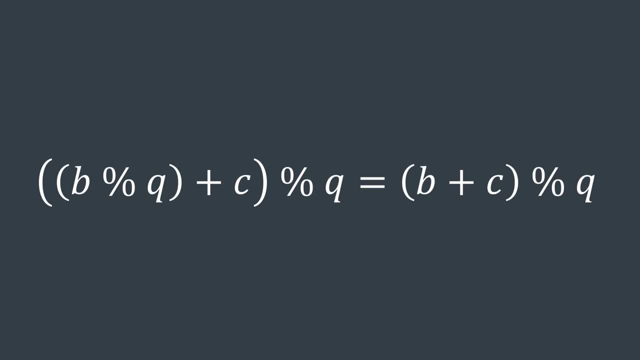 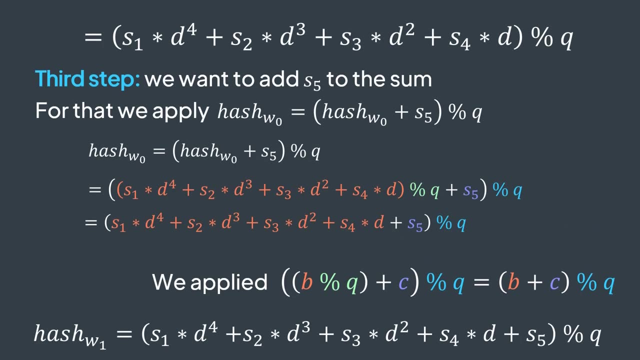 We have this law: b modulo q plus c. all modulo q is equal to b plus c modulo q. b is our actual expression and c is s five, the character we want to add. By applying this law, we can get everything as one. 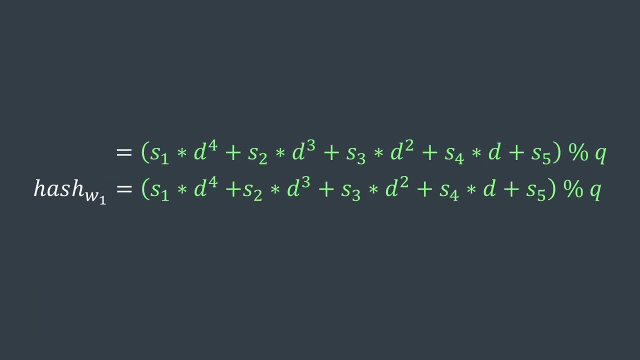 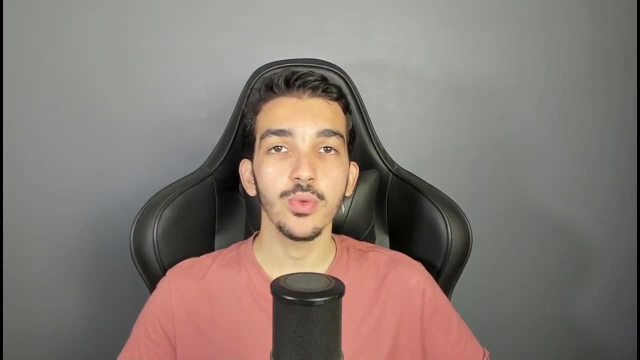 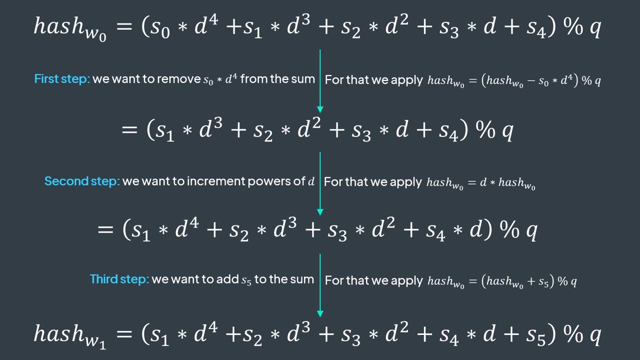 The answer is modulo q, which is the hash of the next window. as you can see, We've been able to get the hash of the next window by applying these three steps: Subtract s zero times d, power four, then putting modulo q, multiplying by d and adding s five. 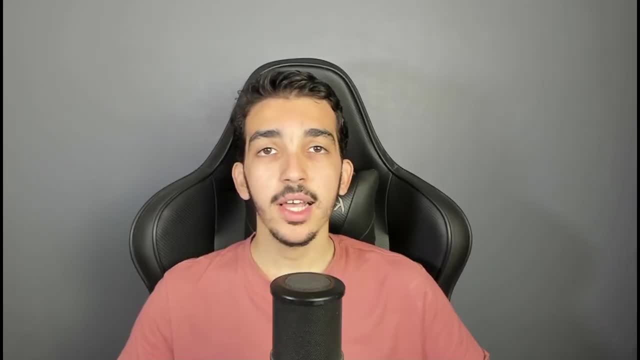 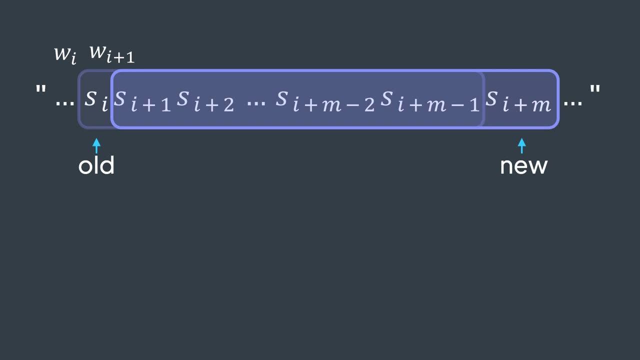 then putting modulo q. Let's generalise. We have the window that starts at index i that consists of the next m character. We can also add in the arrow hexagons We can find the new character on numbers from index i to index i plus m minus one inclusive. So it's hash is si times d. 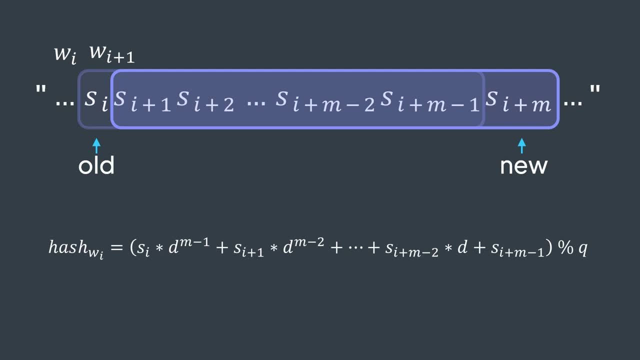 power, m minus one plus s of i plus one times d power. m minus two, and so on until s of i plus m minus two times d power. one plus s of i plus m minus one times d power. zero. all that modulo q. And we want the hash of the next window, the one that starts at index. 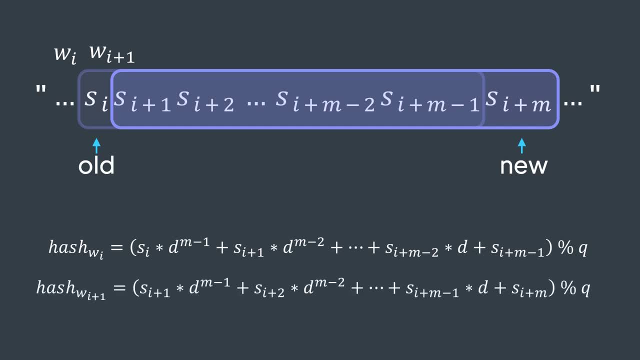 i plus one. Its hash is s of i plus one times d power- m minus one. plus s of i plus two times d power- m minus two, and so on until s of i plus m minus one times d power. one plus s of i plus m times d power. zero modulo q, For that we subtract s of i times d power, m minus. 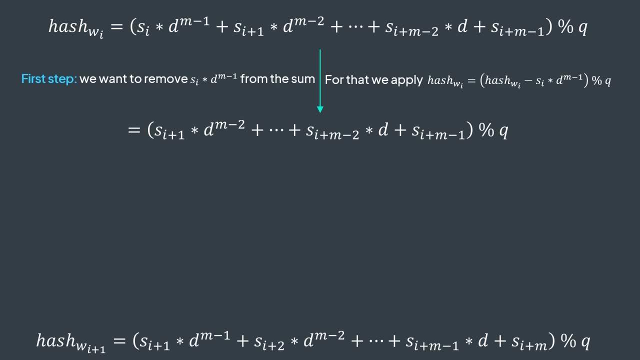 one and set modulo q. we get this result. Then we multiply by d, we get this result. And then we add s of i plus m and set modulo q. We get the hash of the next window. We can even add modulo q for d power, m minus one. 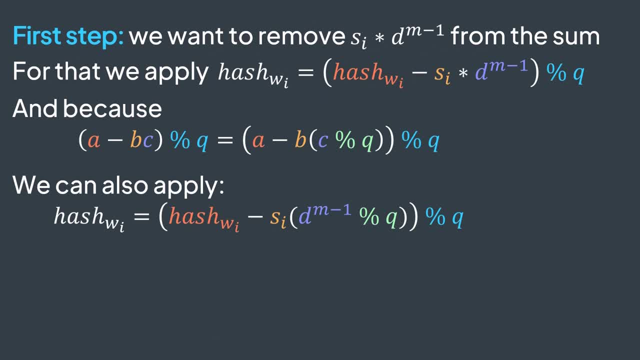 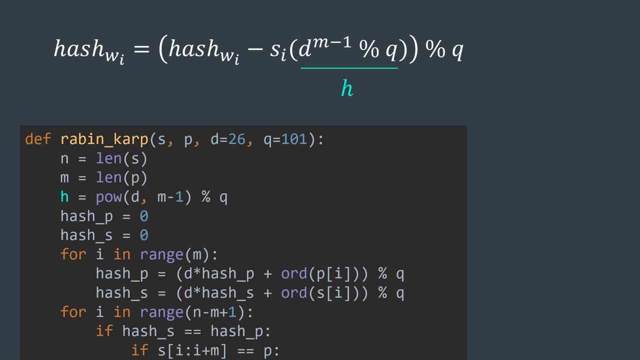 in the first step In code we add a variable h where we store d power m minus one modulo q, to avoid computing it again at each iteration. And, by the way, we should be careful when calculating it: d power m minus one can cause an overflow And after comparing we have 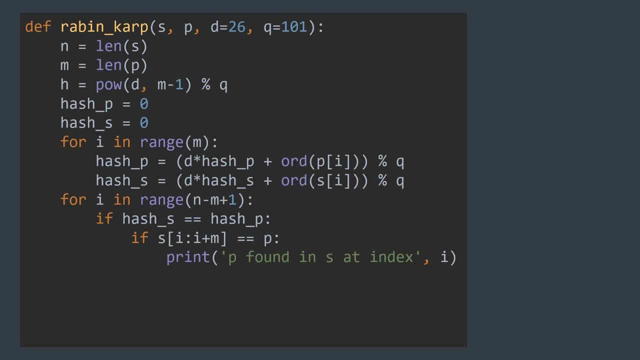 to update it. Note that we don't update in the last iteration because in the last iteration there is no iteration coming after it, so no need to update. We can't even update because there is no new character to add. So we add this condition: We must be before the last iteration. 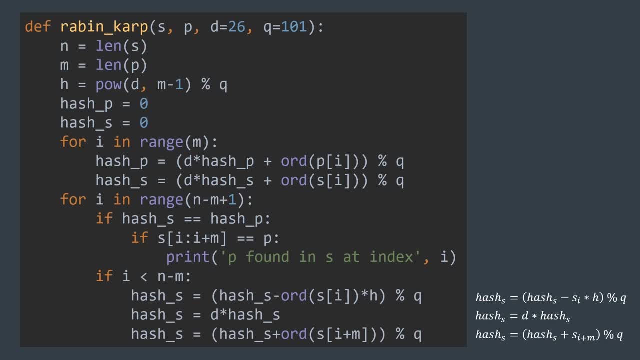 Inside, hash s becomes hash s minus s k of s i times h, all that modulo q. Then we multiply hash s by d And finally hash s becomes hash s plus s k of s of i plus m, all that modulo q And. 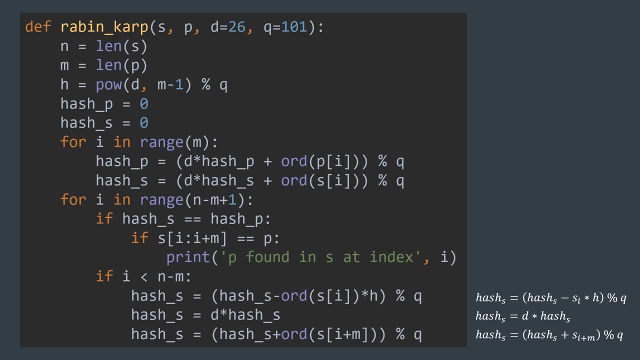 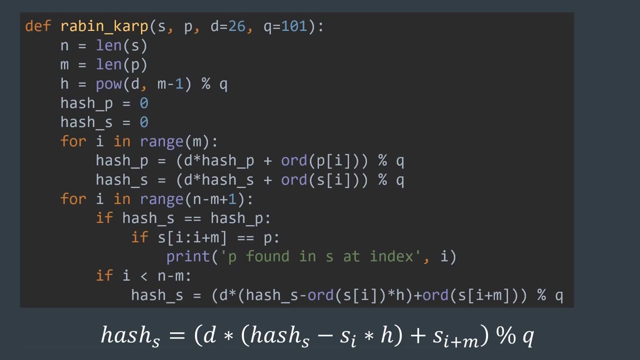 we get the hash of the next window by applying those three steps. We can even combine everything into one operation. Hash s becomes d times hash s minus s k of s i times h plus s k of s of i plus m. all that modulo q. 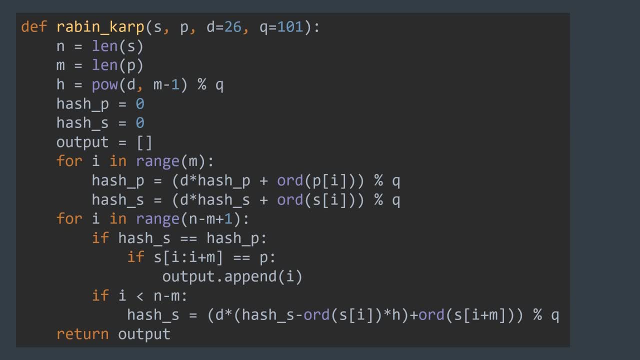 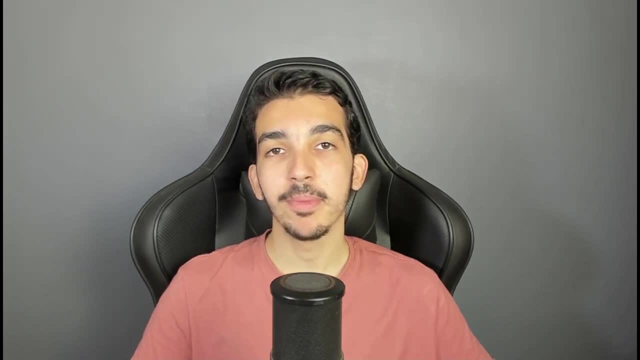 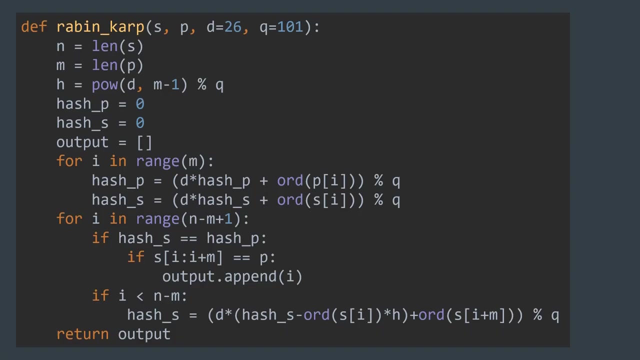 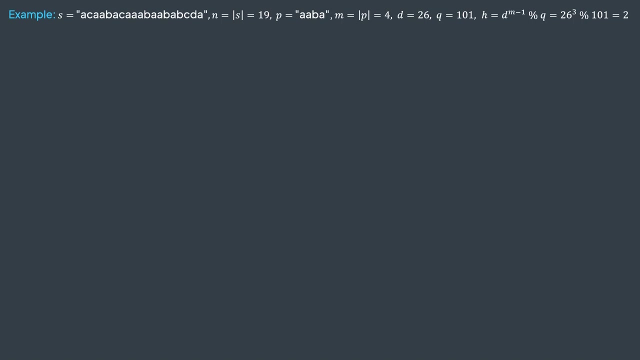 can also store indexes where we find p instead of just printing to be able to return them after as an array. and we got our robin carp algorithm implementation. i hope that math demonstrations wasn't too heavy. let's apply it on this example and see if it really works. m is 4, d is 26, q is 101. 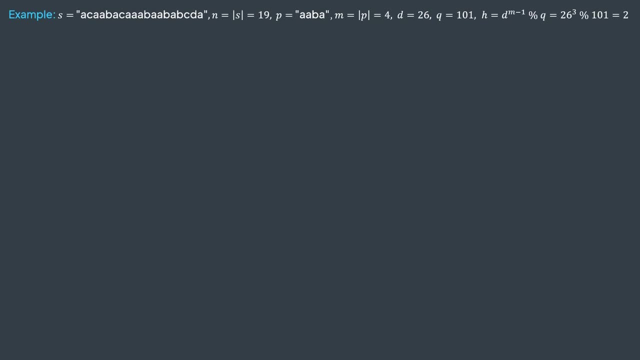 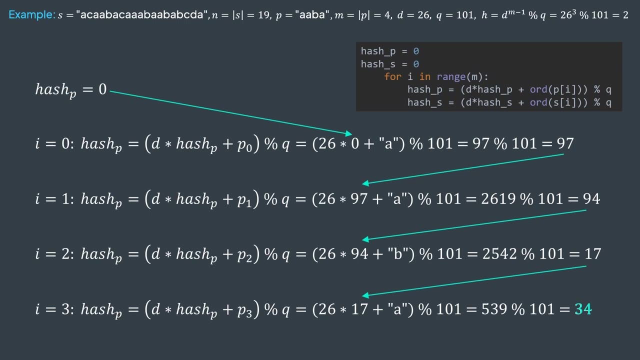 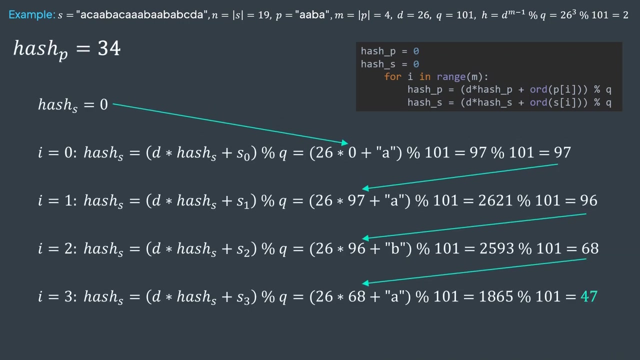 and h is d, power m minus 1, module q, which is 2.. we calculate the hash of p. we start at 0 and apply the operation for each character: we get 34.. same thing for the first window of s, the first four characters, we get 47.. 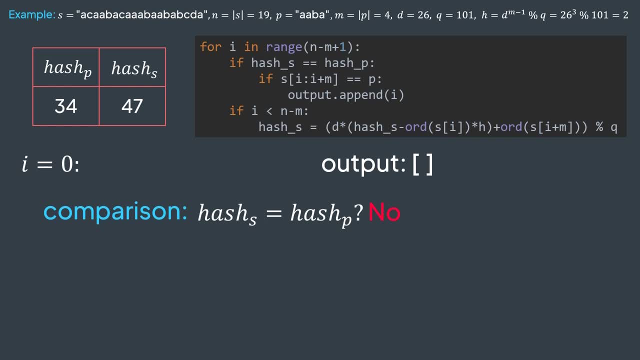 now we start iterations. first iteration: hash s and hash p don't match. we update for the next iteration: we get 13.. next iteration: they don't match, we update, we get 34.. next iteration: here they match. let's double check the window. and p are equal. so we found p and s at index 2.. let's continue, we update, we get 80.. 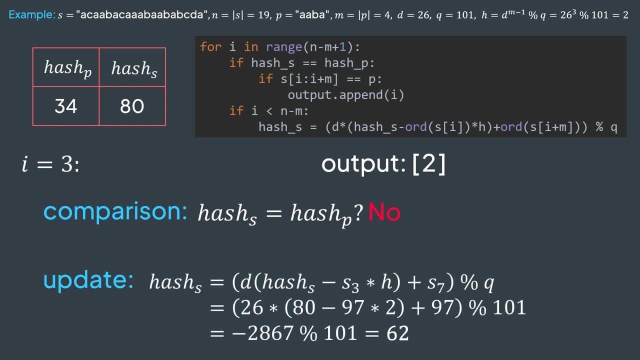 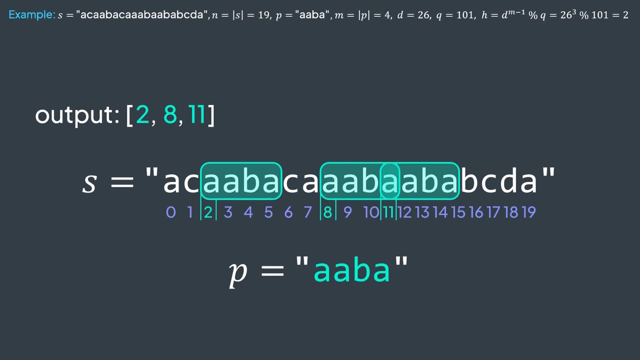 next iteration: no match. we update, we get 62. and it continues like this for remaining iterations. we get 32.. the result is that we can find p and s in three locations, at indexes 2, 8 and 11, which is true. our algorithm worked. last thing, to talk about time complexity, because after we did all, 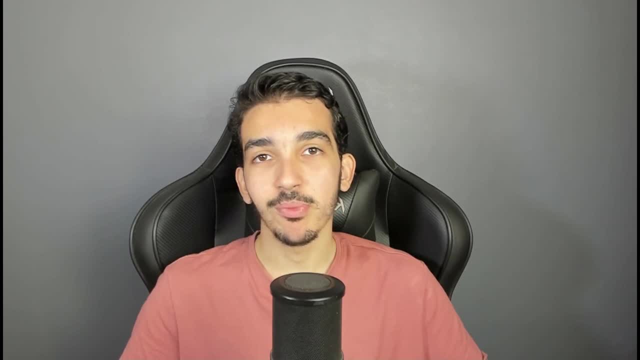 of this, we obviously ask ourselves if we got an improvement. this is what we will see. first, we have a loop that traverses m characters while we're operating through it. first, we have a loop that traverses m characters while we're operating through it. 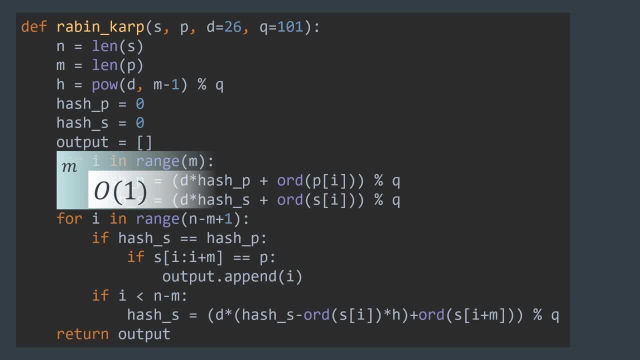 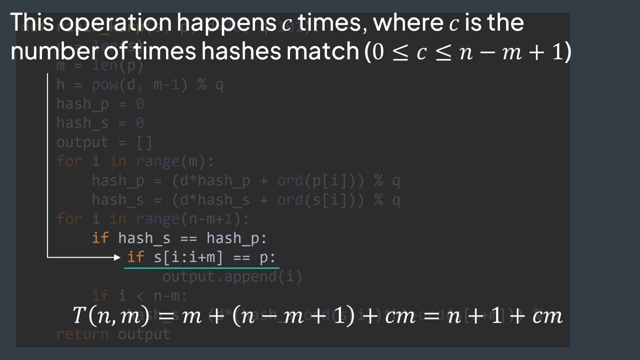 characters while doing O operations. Then we have a loop that traverses indexes. All operations are in O, except comparing the strings, which costs m. However, this operation doesn't always happen. it happens only when hashes match, And hashes match in two cases: when we find p and when there is a collision In the worst case. 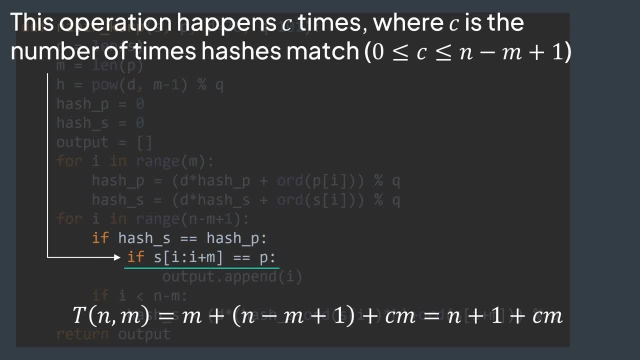 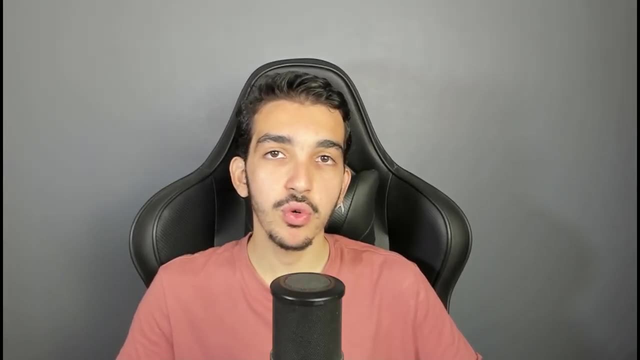 c can be equal to n-m plus 1, hashes match at each iteration. For example, when we have a very bad hashing function or p appears at each index, we get an O time complexity. But with a good hash function most of the time we'll probably have no or very few collisions. 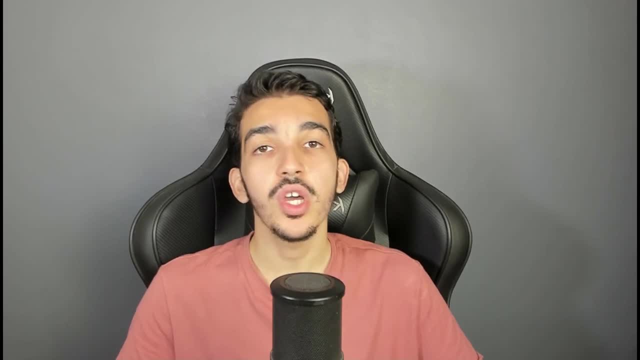 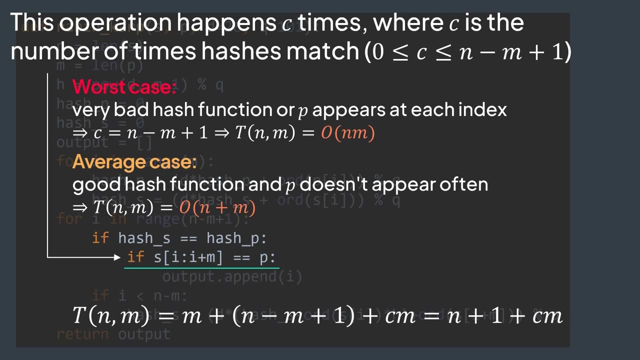 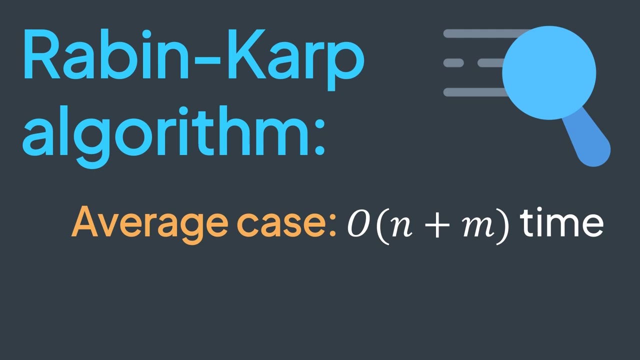 Same thing for appearances. the number of appearances is usually way smaller than n, if not zero. So we can say that in the average case Robin-Karp algorithm has an O time complexity way better than O, But we still have O time in the worst case. 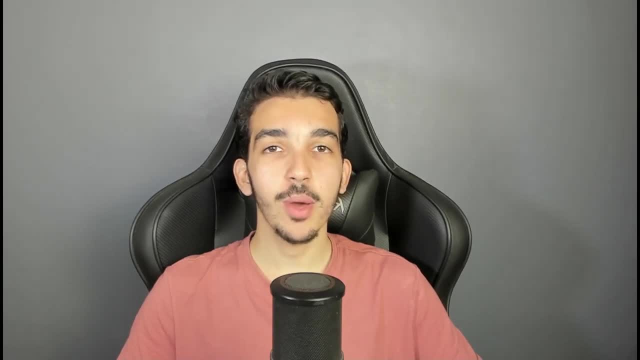 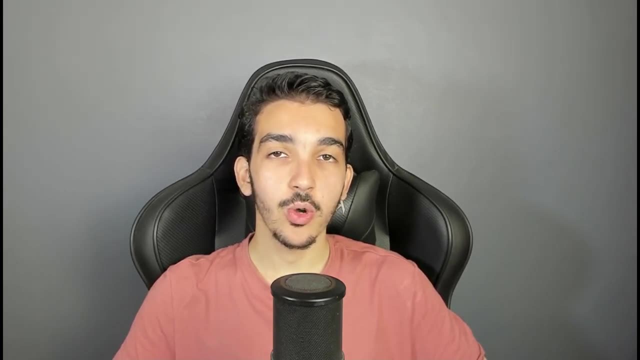 We've come to the end of this video. I hope that you understood how does the Robin-Karp algorithm work. If you enjoyed, like and subscribe to the channel, or you can buy one of the inside code courses that you can find below in the description. See you in the next video.